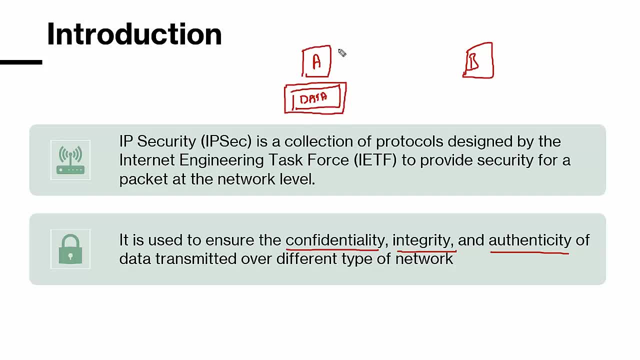 data is basically protect with the key. so we have encrypt the data, so data will remain encrypted throughout the journey and it reach B and B will basically use the same key to decrypt the data. so by this way, it offer the confidentiality. it also offer integrity, authenticity, how we'll discuss in a later stage before. 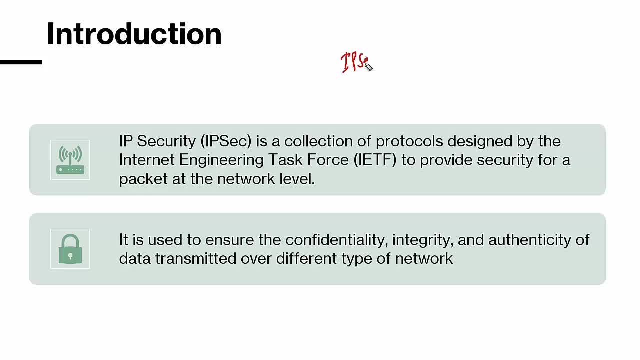 we're going to discuss about IPSec in detail. let me tell you the IPSec family. in IPSec, we basically have a three important component. one is basically called as a protocol, one is basically called as a mode and one is basically called as a key exchange. so when you're talking about the protocol- protocol- we 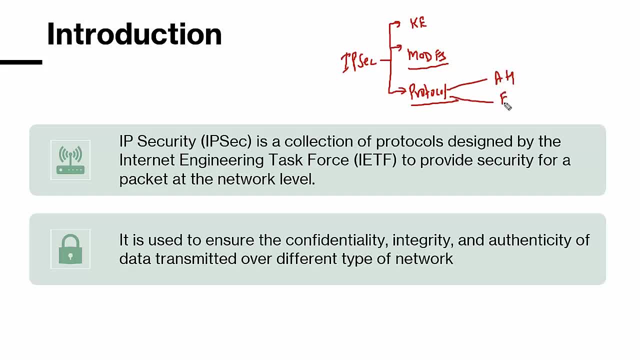 have a three type. one is called. two types are A, H and E S P. when you're talking about modes, we have a two modes in IPSec. one is called as a transport mode and one is basically called learning performance as a tunnel mode, and the key exchange is basically achieved through ISA, KMP, OKLE and SEA SME. 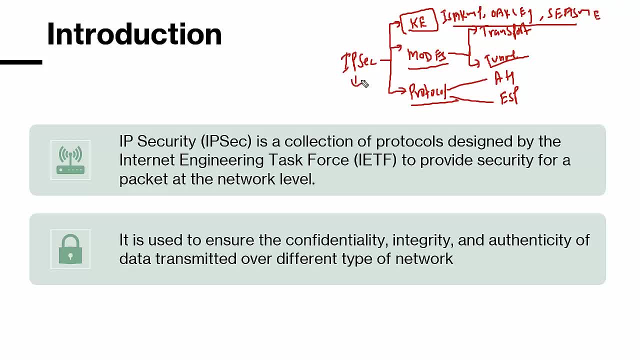 So these are the some of the parameters we have. for data encryption, it basically use AES and for the key exchange, it use Diffie-Hellman. along with that, for the hashing is basically use the SHA. so this is basically the primary goal of IPSec, or primary component of IPSec. 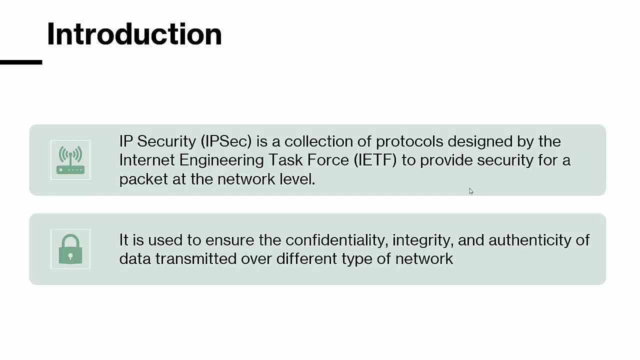 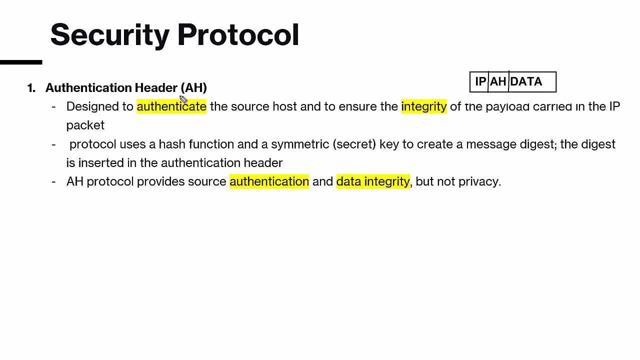 ultimate goal. whatever the data we are sending over the network, it should be protect from unauthorized disclosure, unauthorized modification and giving an assurance that it is coming from the right source. so the first thing we are going to discuss in the IPSec is the protocols. so the first protocol that we are going to discuss in IPSec is AH. so AH is designed to. 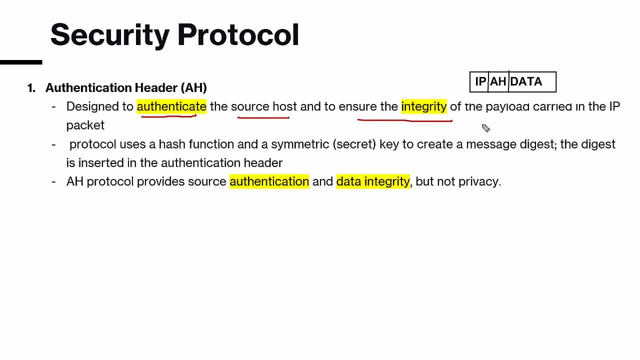 authenticate the source host and ensure the integrity of the payload carried in the IP packet. how, example, like we have a system A and we have a system B. okay, so this is basically my data. so if you see the statement here, it is clearly mentioned: the protocol use a hash function. so what we use to do is we create a hash value of the. 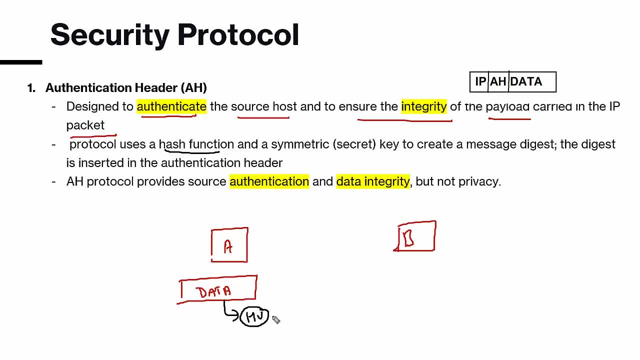 data, we generate the hash value. hash value is represent the integrity state of data. so example: right now the time is basically 638.. So at 638.. The data was formed and this is the hash value of the current state of data. is it clear? and then this hash is basically encrypted by the symmetric key and we append the AH. 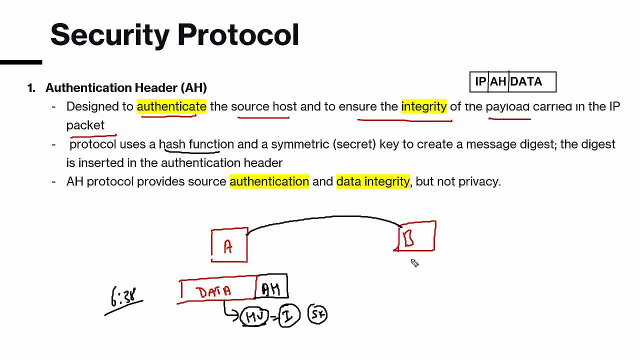 header as a signature into the data and when we send this data to B, when we receive the data, they will see the AH header. so first AH header will be decrypted by the secret key, then they get the hash. so that is an assurance that this is coming from the A, because B already. 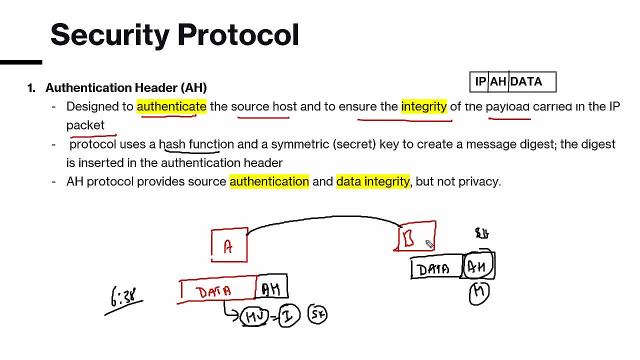 have that same session key which A has, so that give the assurance It came from the A. now we have to check the hash value. by check we checking the integrity state. so we scan the data and check for the hash and compare this hash with this hash. so 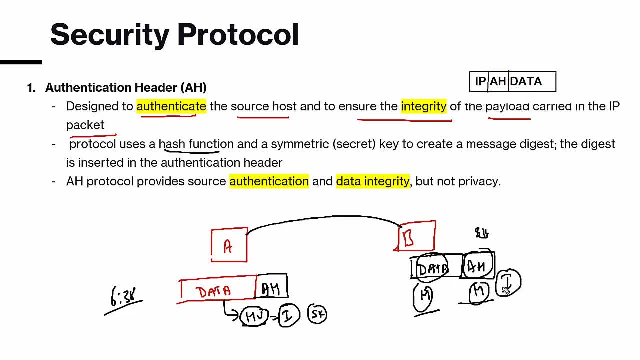 if it same, it mean it gives also the assurance data came without any unauthorized modification. so that is why I called protocol, use a hash function and symmetric key to create a message digest which is called hash, and insert into the authentication header. that is why AH primary of authentication and data integrity. 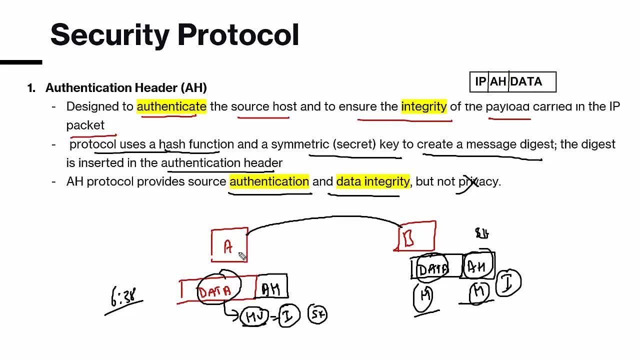 But not a privacy, Because anyone can able to read the data. is it clear? because when we when A sending a data to B, okay, so example: someone is sending a data, okay, so attacker is here, he can basically intercept the data and easily for the user to read the data, it doesn't matter for them. 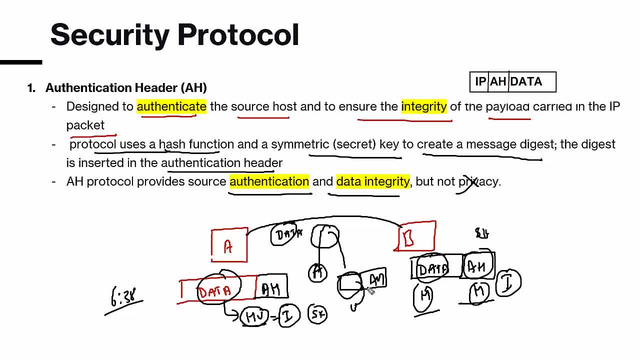 what is AH, is it clear? but if we modify the data and resend, B can able to identify. this is not the same data which came from A because it is encrypt by the unique keys. So AH primarily offer the authenticity and integrity of the data state. but if you looking 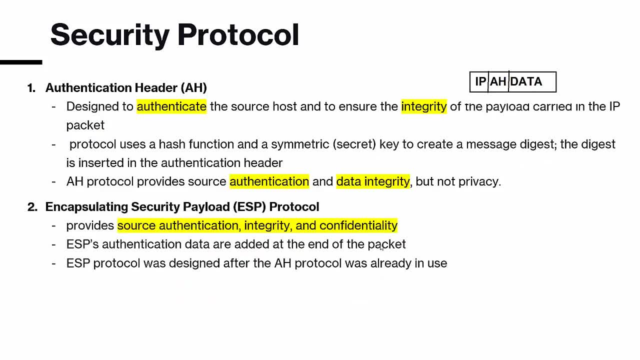 for the complete solution, end to end solution. then we have a ESP, which basically provide the source authentication, integrity and confidentiality. so, example, like we have a system A, we have a system B. this is basically my source. this is my destination. So far, what we have learned is we have a data to give an assurance. it is coming from A and 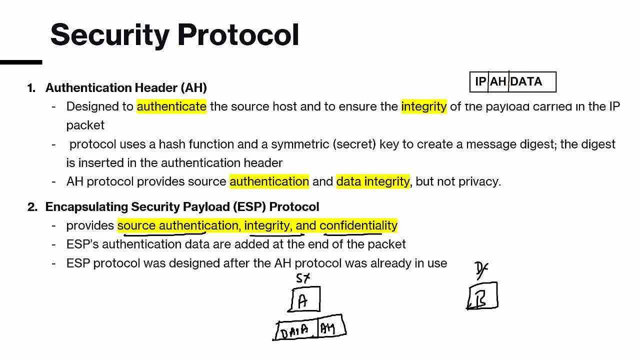 with the integrity state, we add the AH header, but then what happen is they basically encrypt the entire data into new packet and then it basically sending that encrypted data over the network. Now, if there is attacker, if you monitor any capture, this they cannot able to read anything. 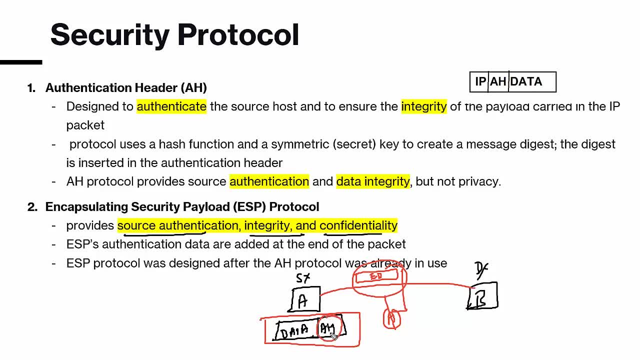 on that. so it already having a authentication header which providing the authenticity, which capture your integrity, hash value, which provide the integrity and also encrypt the entire data. So it provide the source authentication, Integrity and confidentiality. So ESP authenticating the data are added at the end of the packet. 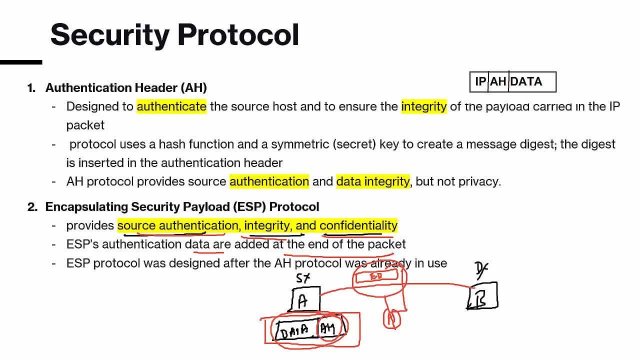 So ESP protocol was designed after the AH protocol was already in use. So first we introduce the AH and when we discover the issue in the AH, then only we introduce the ESP. So same example we have: we have a data, then we have a AH header and then we have a IP. 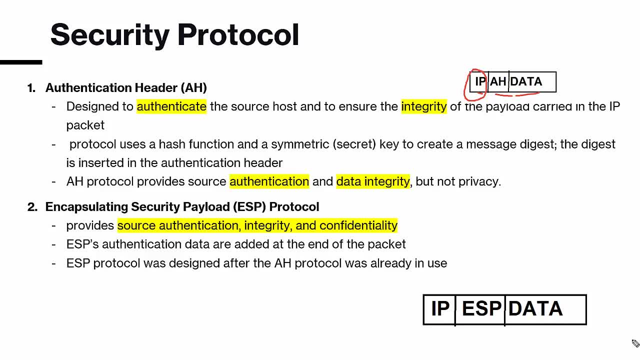 This is the external IP which is used by the router, by which they routing the information. but in this case, data then encrypt the data, Then we adding the external IP By which the routers can able to communicate. So, if you go by the security protocol comparison. 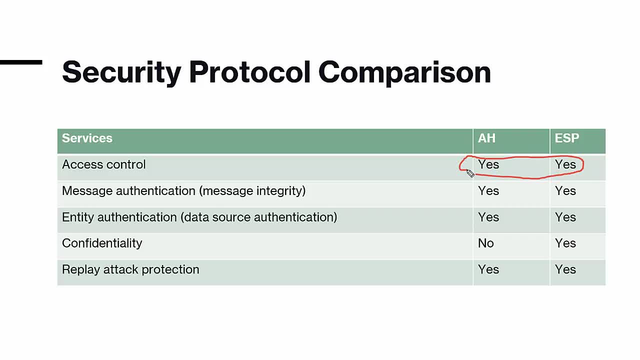 Access control offer by both AH and ESP. Message authentication offer by both. Entity authentication it mean data source offer by both. but confidentiality AH doesn't offer. It is basically offer by ESP. Replay attack protection offer by both. because when we say system A and system B and there 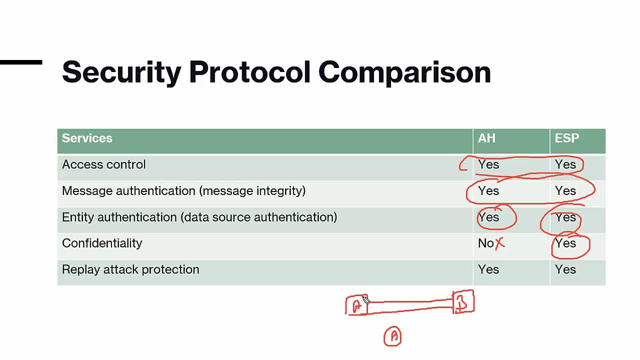 is attacker, B is sending any data, B is asking for the password and he is sending something, So he will capture and resend. that is not possible in the case of IPSec, because every packet has a unique packet header by which we can able to prevent the replay attack protection. 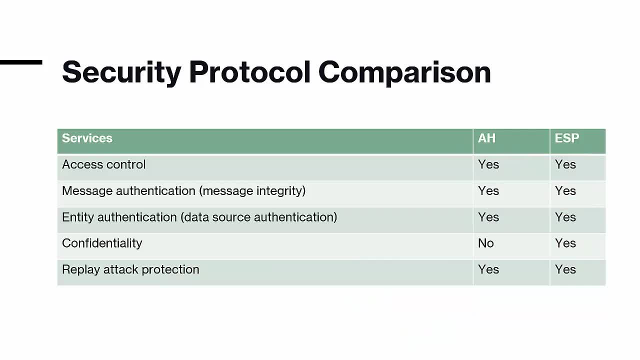 So it solution offer by the both AH and ESP. So today IPSec is also used in a Microsoft. It is used in a Linux in a form of policies. How example, like we have a domain controller And here we have a switch, We have a system A, We have a system B, We have a system C And we have a system D Now 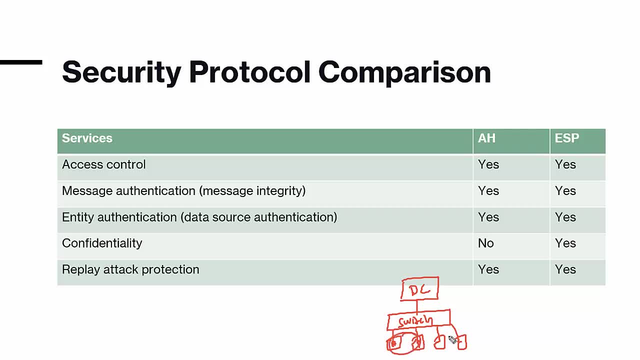 you want to ensure that A can only communicate with B And you want to ensure C can only communicate with D. So from D- C we can create a IPSec policy And by which we can ensure that A can only communicate with B. B can only communicate. 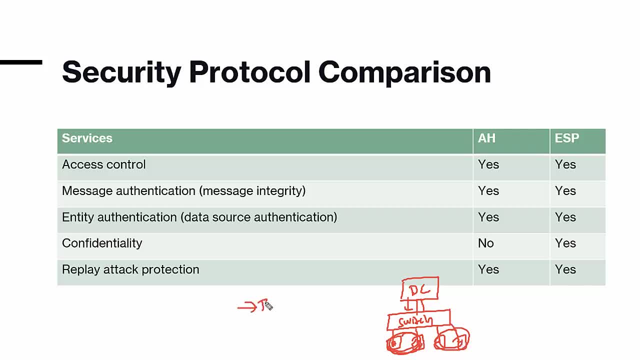 with A, C can only. So this is basically called as a feature called IPSec filtering. Another important feature which IPSec offer is port security. So this feature is called as a feature called IPSec filtering- port security. what is port security? is suppose we have a server here, web server, so from a domain. 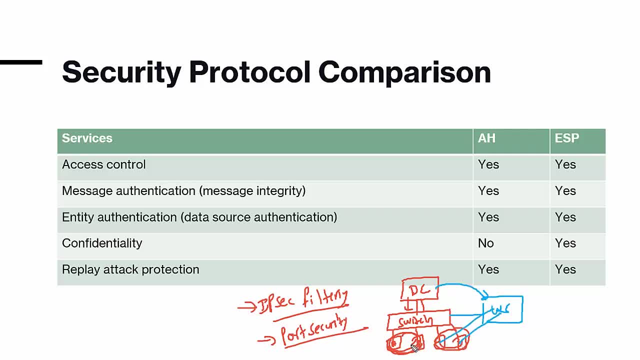 controller. we apply the IPSec policy that they can able to access. they can able to access by a port number 80, but if they try to ping on ICMP that will be blocked. so IPSec offers this kind of an access control. is it clear? but primary into the introduction of IPSec was a data security. 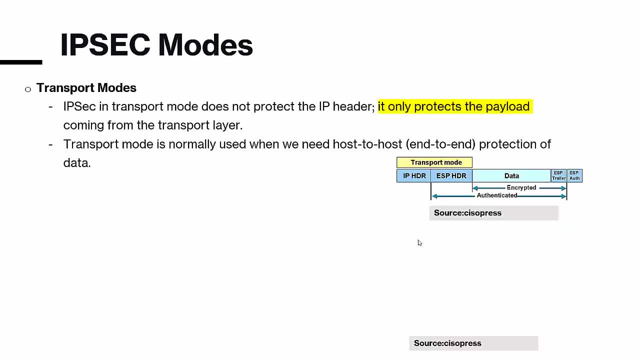 which need to be over, send over the network. now, when we talking about IPSec, in IPSec we have a different modes. so in IPSec we have a different type of mode. the first mode is called as a transport mode. IPSec in transport mode does not protect the IP header, it only protect the payload. 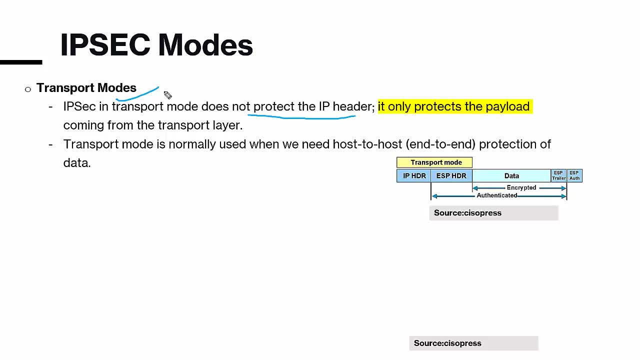 coming from a transport layer that is basically called as a transfer mode. it is also called as a and to and encryption. so this mode is used when we need to communicate between host to host you. example, we have a System A and we have a System B. okay, here we have a firewall, here we have a. 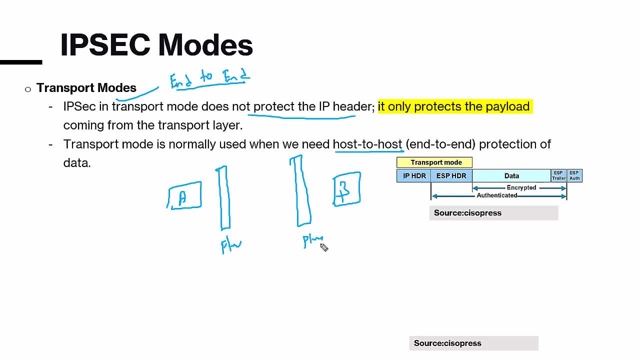 firewall. so this mode is basically happening between and to and host, so between A and between B this encryption happen, so in which they only encrypt the data, A, H and ESP's: A, H is basically visible, so it's only encrypting a data, but high IP header is basically visible. you can see we 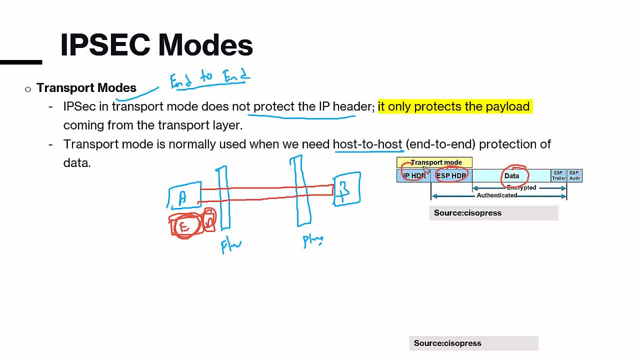 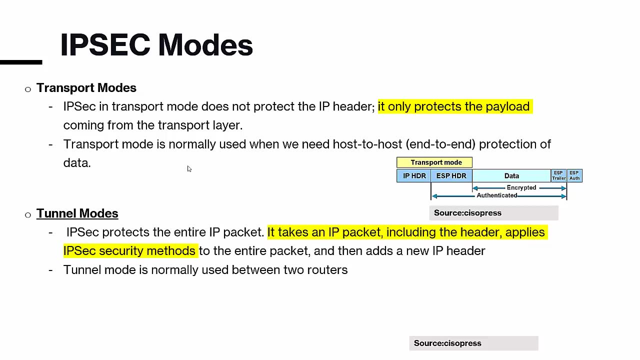 have a data, ESP header, IP header- okay. so in this case they basically encrypt the data, but header is basically visible and that is why it is used between the two hosts. but between the two firewalls we basically use a tunnel mode so it protect the entire packet. it take the IP packet including the header and basically apply. 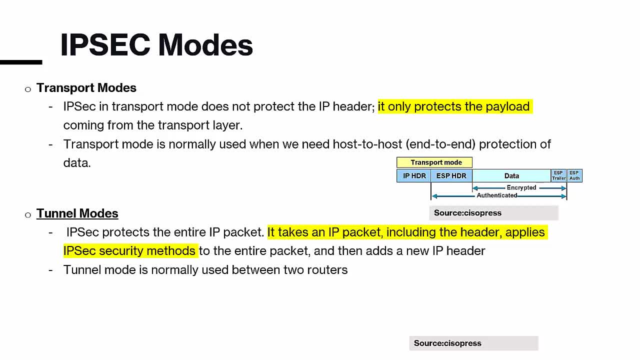 the IPSec method to encrypt the entire packet and then they add a new header. so it is basically happening between the two routers. so if you take example, the same example we have- so this is basically called as a transfer mode, and between these two routers we basically 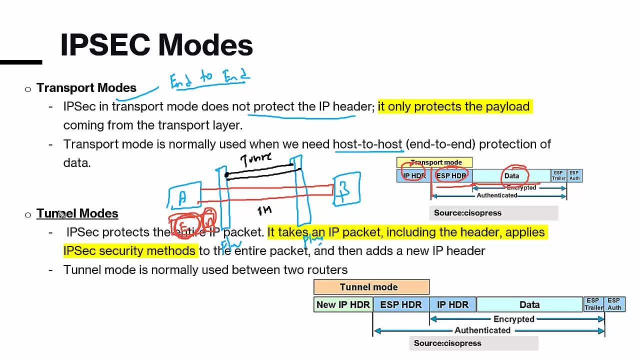 have a tunnel mode. that's where tunnel mode is called as a link encryption, which is happening on the layer 2, and transport mode is basically happening from application to transport layer encryption, which which is also called as a application level encryption, or and to and encryption. okay, so, if you can see the 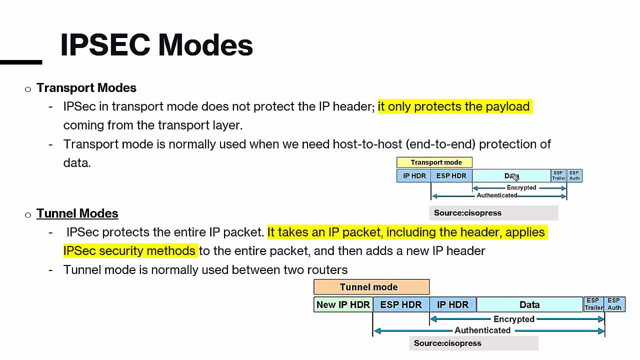 packet, header, size and types. so we have a data which is only encrypted. rest is basically visible. but in this case data is encrypted along with the ip header is also encrypted. so definitely, tunnel mode is basically offer better security. now in which condition we use tunnel mode. so company want to create a secure tunnel between its headquarter and remote office. 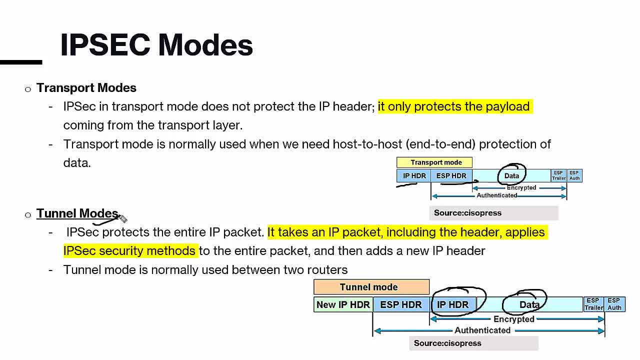 they would use tunnel mode. the government agencies: they want to create a secure tunnel between its headquarter and embassies around the world. they will use tunnel mode. the bank want to create a secure tunnel between the headquarters and atm. they will basically use the tunnel mode. along with that, we have a case studies where the transport mode is used. example: 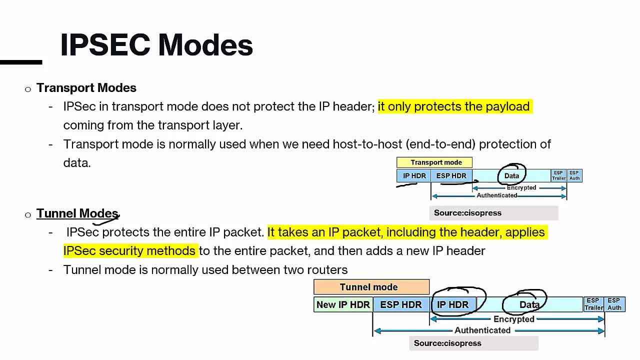 user want to securely access the work files from the home, they will use transport mode. the user who want to securely connect to the remote desktop, they will use transport mode. or user want to securely ascend an email would use the transfer mode. but the question is, what is a key by which they encrypt the data? so we have a third important component in the IP sec. 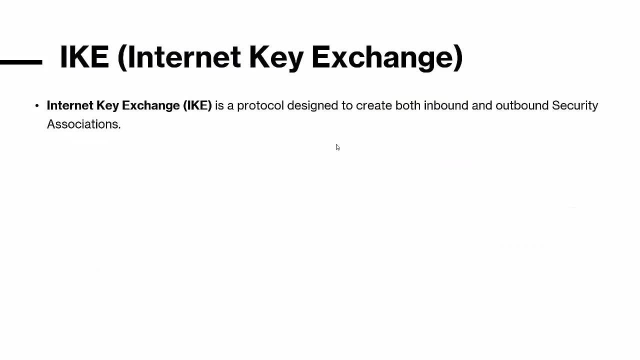 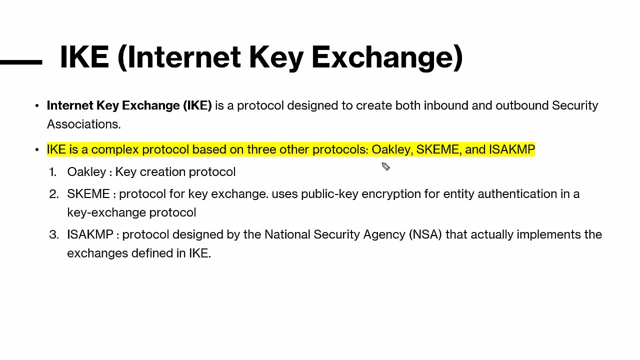 which is called as a IK internet key exchange. so it is a protocol designed to create both inbound and outbound security association. so IK is basically the complex protocol which is based on the other three protocols. one is basically called as Oakley, one is called as a skimmy and 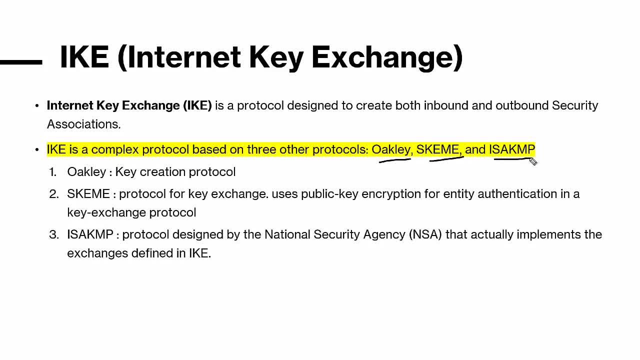 one is basically called, as is a KMP. so first is basically called as a Oakley. Oakley is basically called as a key creation protocol, okay. so you can say we have a stadium, okay, in which we need to play cricket. so Oakley are the players you can say okay, who want to play a cricket which. 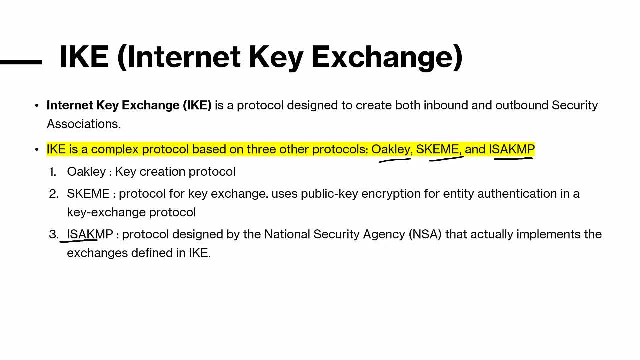 is used with the is a KMP. I see can be provide the infrastructure, like what is the mode and what is the key and what is the algorithm we have to use. but when you're talking about skme, skme basically stand for secure key exchange mechanism, so it was an alternate. of- is a KMP. so today, if you